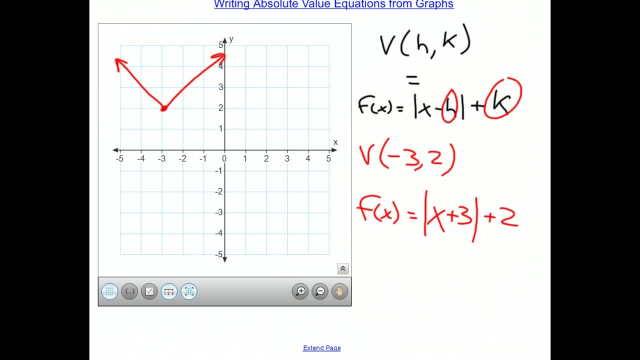 And there we have it Right. this tells us that our graph should be shifted to the left 3 and up 2, precisely where we are Right. not too challenging, Let's take a look at another one. So let's take a look at this graph. 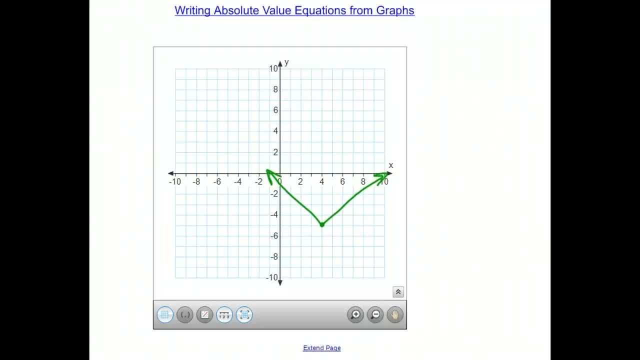 We have certainly another translation. Okay, the vertex has certainly been shifted. Where's the vertex? Well, again, it's as simple as locating where it is in the coordinate plane. What's the x coordinate? We know the x coordinate is 4.. 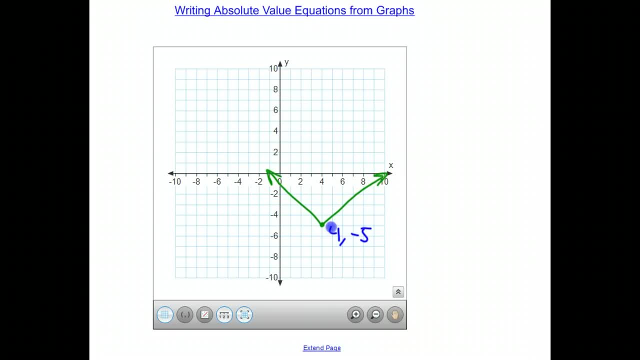 We know the y coordinate is negative 5.. Right, so our vertex is: So our vertex is here: at 4, negative 5.. Can we plug this into our equation? We should be able to: Right, we have: f of x equals the absolute value of x minus h. 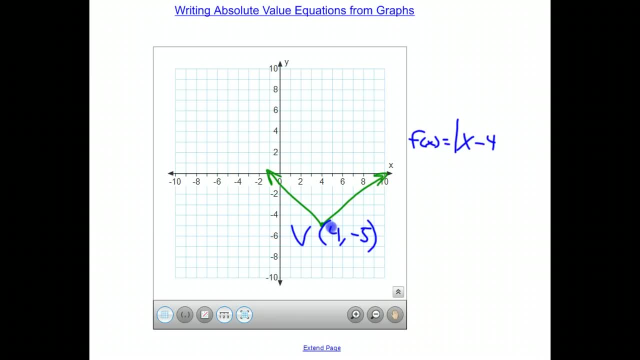 h here is 4, so it's x minus 4, plus k plus a negative 5.. And just to keep it simple, I'm just going to write negative 5 there. So there's our equation. Fairly straightforward and it's not really that painful. 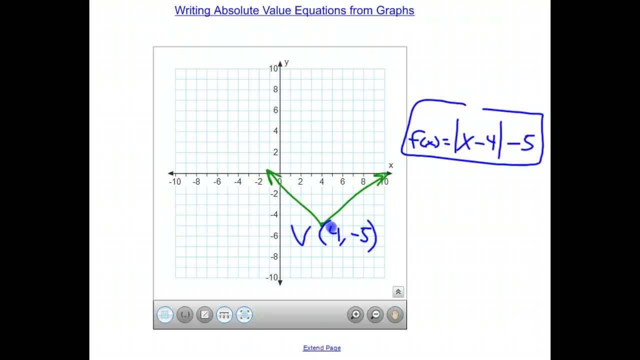 If you can look at a graph and find out where the vertex is, you should be able to give the equation. Okay, I'm going to give you one more tricky one and we'll go over it together. Then I'll give you a few on your own to practice. 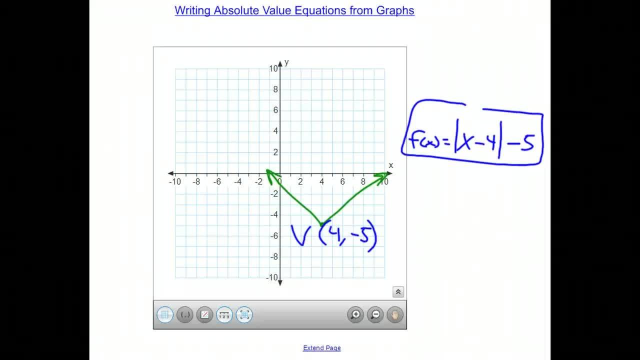 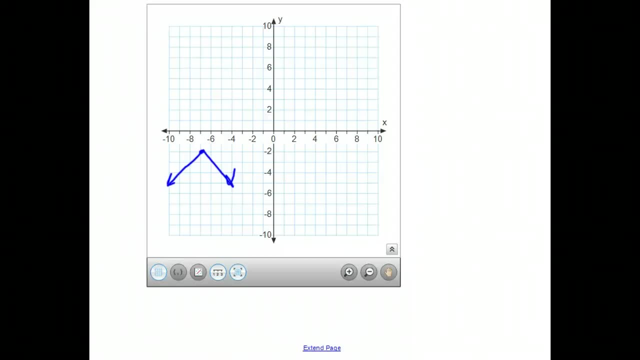 and we'll talk more about this in class tomorrow. In this graph, there's slightly more going on. First of all, what do we notice that's different? What do we notice that's different? What do we notice that's different from this graph? 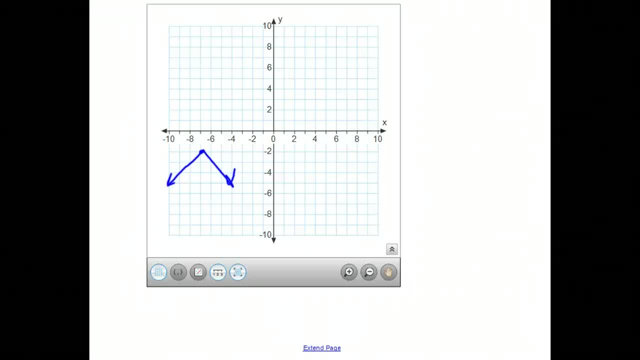 than in the previous two graphs that we talked about in today's screencast. You all should be able to tell that this graph is a reflection which tells us what. It tells us that there's going to be a negative sign in front of the absolute value. 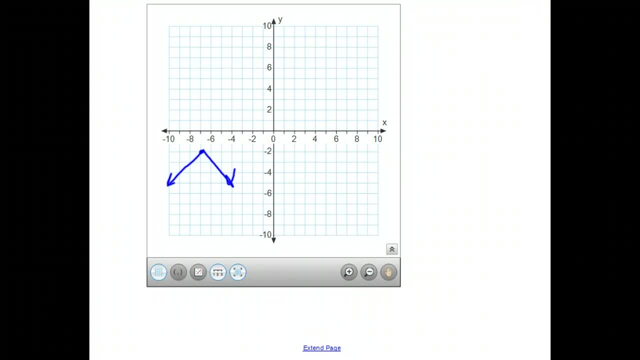 So we actually find this graph the same exact way. All we need to do is find out where the vertex is. So here the vertex is going to be the x coordinate, which is negative 7.. Fairly easy to find. The y coordinate is negative 2..